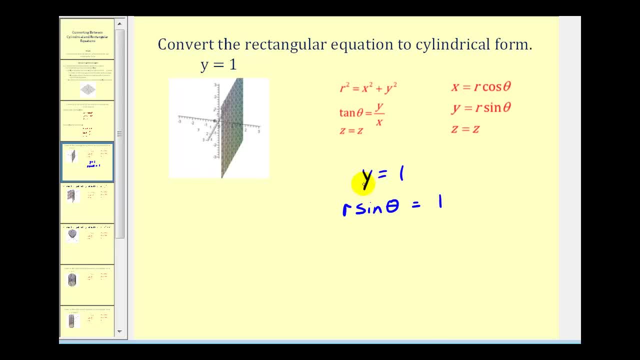 Now, typically when we have a cylindrical equation, we want to solve it for r, So let's go ahead and divide both sides by sine theta, So r is equal to one sine theta, but we can rewrite this to eliminate the fraction, as r equals cosecant theta. 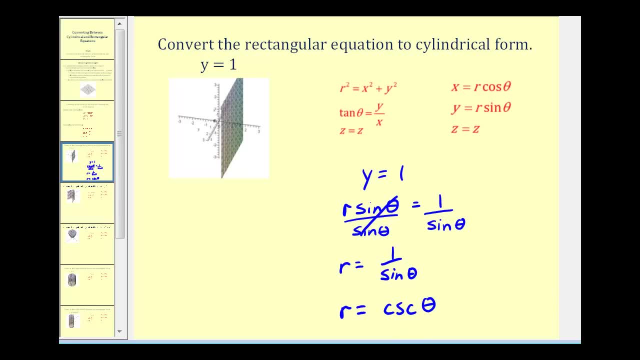 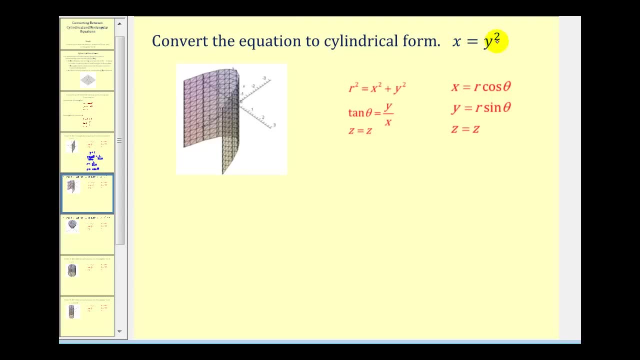 Remember: sine and cosecant are reciprocals of one another. Let's go and take a look at another example. Here we have the equation in rectangular form: x equals y squared, and here we see the graph of the surface. Again, we want to eliminate x's and y's. 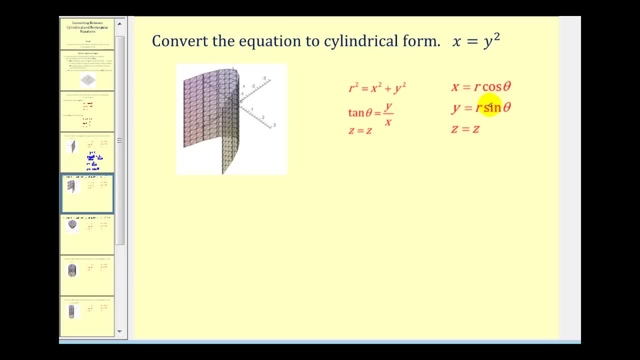 by introducing r's and theta's. So using these two equations here we can replace x with r cosine theta and we can replace y with r sine theta, So we have r cosine theta, and then we have r sine theta squared, Y squared, So we'd have: R cosine theta is equal to R squared sine squared theta. 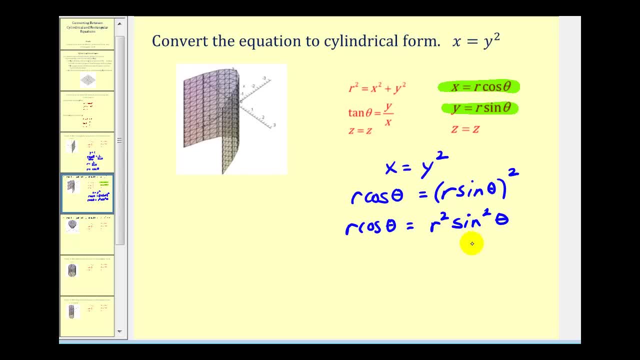 Now again, we typically want to solve these equations for R. So if we divide both sides of the equation by one factor of R and then, sine squared theta, we'd have an R on the right side of the equation. So this simplifies, this simplifies: we're left with R on the right side. Here the 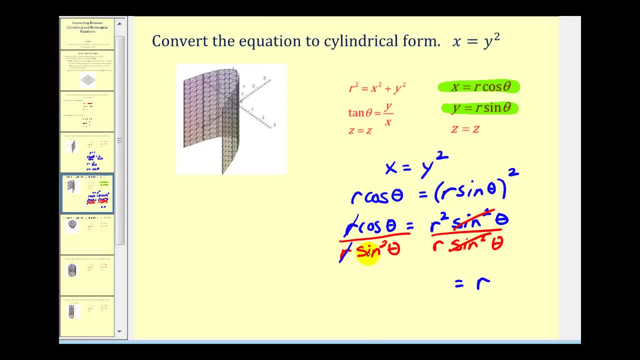 R's simplify out and we're left with cosine theta over sine squared theta. Now I'm going to go ahead and write this as cosine theta over sine theta. and then we have one more factor of sine theta in the denominator. I'm going to write: 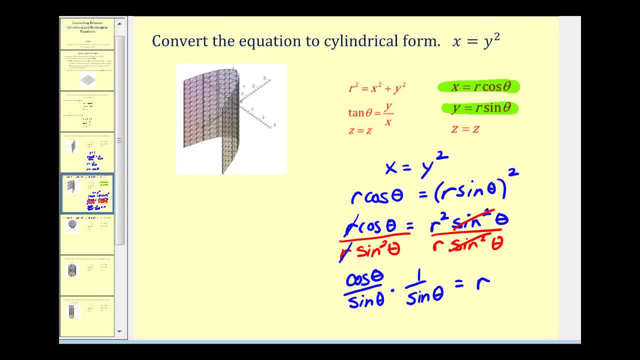 So we can rewrite this as one over sine theta. Now the reason I'm going to do that is I know that cosine theta over sine theta would be cotangent theta and again one over sine theta would be cosecant theta. So we could rewrite this as r equals cotangent theta. 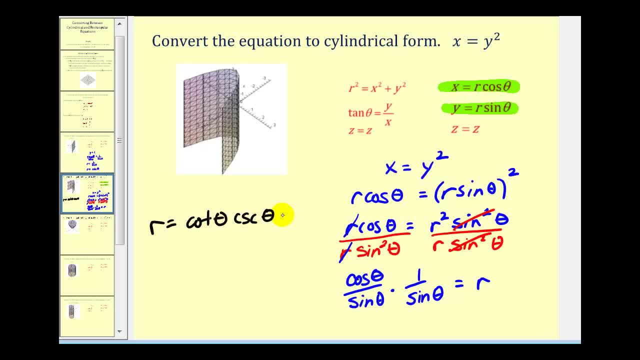 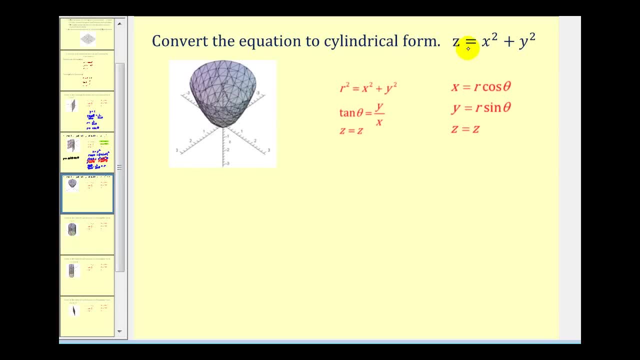 cosecant theta. Let's go and take a look at another one. Here we have the graph of z equals x squared plus y squared. We want to convert this to a cylindrical form. So the z is okay, but we want to eliminate the x's and y's. 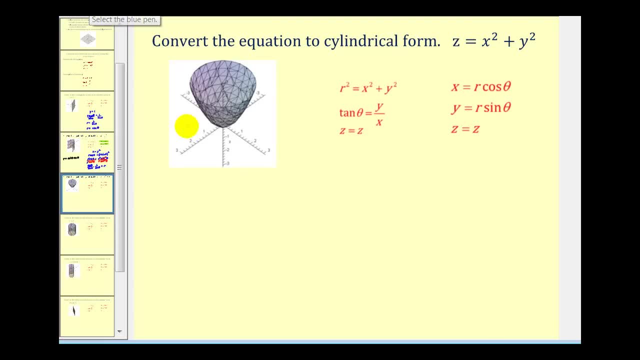 and replace those with r's and theta's, And I always like to see the surface. so here we have the graph of the surface on the left. Now, this one may look like it's going to be a lot of work, but in fact it's actually the easiest one. 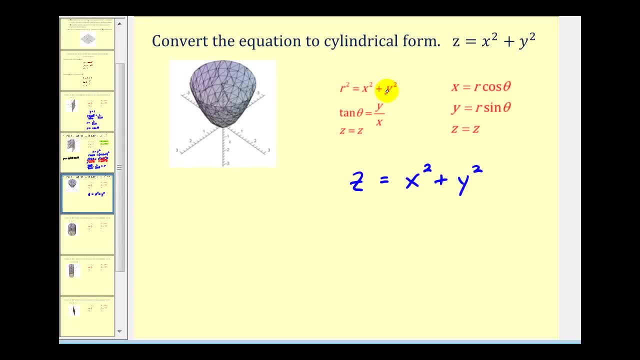 because, looking at all of these equations, x squared plus y squared is the same as r squared. So this is the graph of z equals r squared using cylindrical equations. Now let's go ahead and convert some cylindrical equations to rectangular form. So here we have the graph of r equals two. 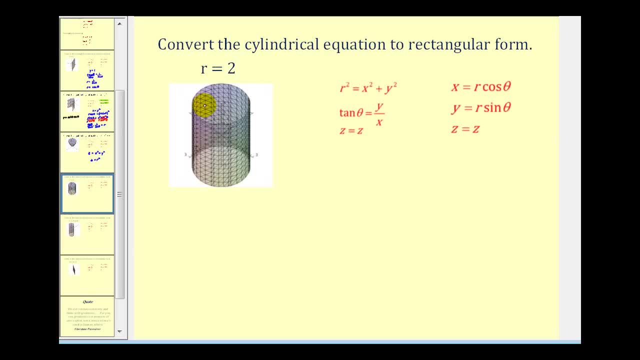 which is a circular cylinder. When we're doing these conversions, we want to eliminate r's and theta's and replace them with x's and y's. So if we take a look at this equation, r equals two, since we know that r squared is equal to x squared. 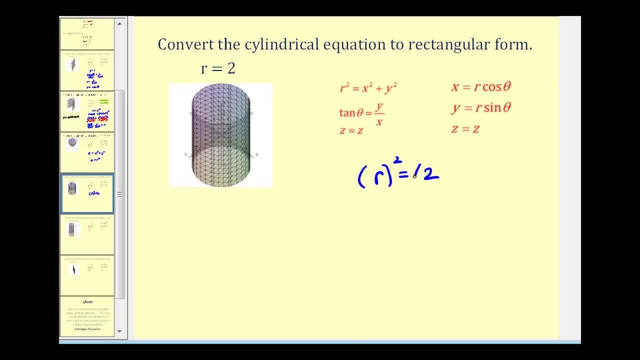 plus y squared. we could square both sides of this equation. That would give us: r squared is equal to four, and now we can replace r squared with x squared plus y squared, And since this equation does not contain r or theta, it is now in rectangular form. 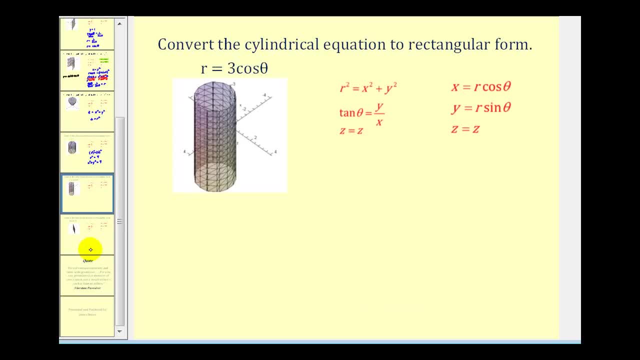 Let's go ahead and try another. Here we have r equals three cosine theta. Again, we want to eliminate the r and the theta by using these equations here, As in the previous example. if we had an r squared here, that would be helpful. but instead of squaring, 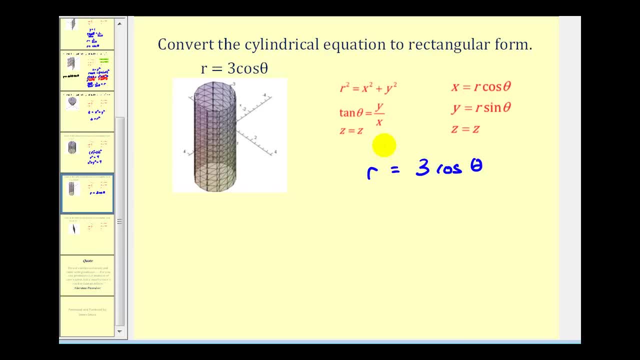 both sides of the equation. this time we'll multiply both sides by r, So we'd have: r squared is equal to three r cosine theta. And now we can replace r squared with x squared plus y squared, And on the right side we have three r cosine theta. 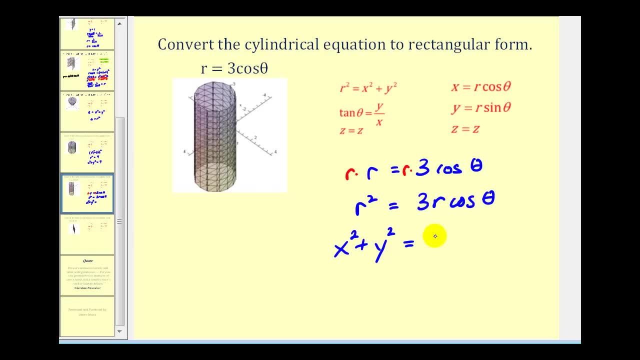 but r, cosine, theta is equal to x, so on the right side we just have three x. Now you might be asking: why don't I multiply both sides of the equation by r here And on the previous example? if I were to square both sides,